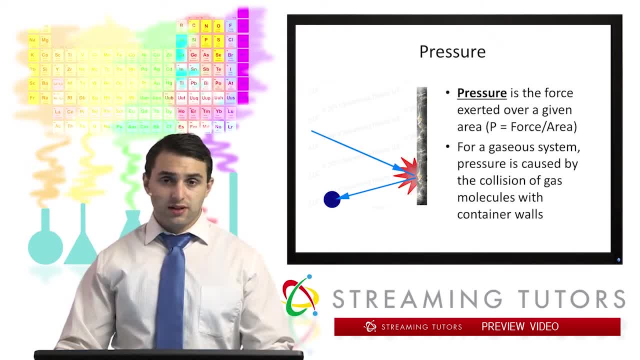 the pressurethe force of individual gas particles on the walls of the container that a gas is in. So when a gas particle hits the wall of a container, it applies a certain force, And the aggregation of all gas particles colliding with the container walls is what gives rise to the pressure of a gaseous system, as you see in this little image over here. 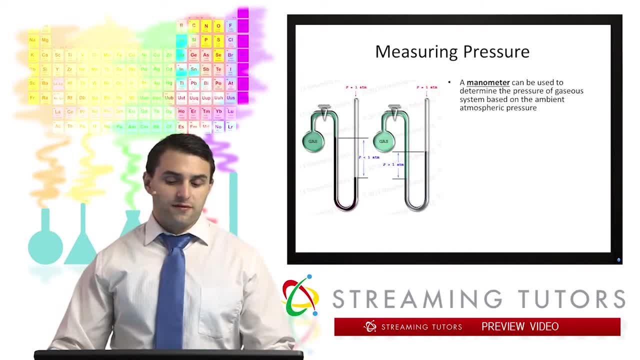 So if we want to measure pressure, we can do that in the following way. So this device here is called a manometer and it's just a way to determine the pressure of a gaseous system. We have our gas in our container on the left and then we have the system exposed to atmospheric pressure. 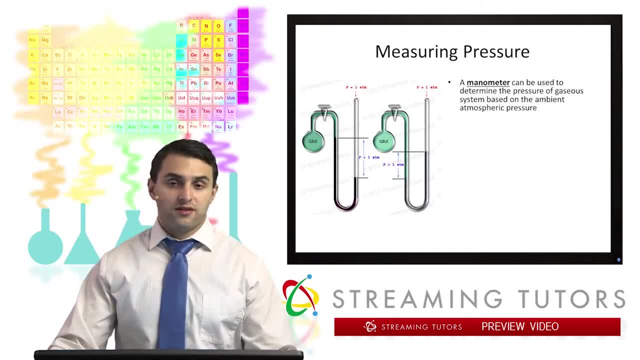 And so we're going to measure the pressure of a gaseous system based on the comparison of the system's pressure to the atmospheric pressure, And the way that happens is we have mercury in this tube, in the U-shaped tube, And as pressure changes between atmosphere and the system, that mercury is going to be pushed either towards the container or towards the end of the tube. 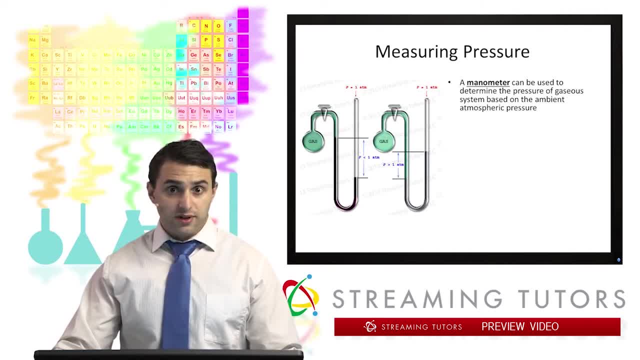 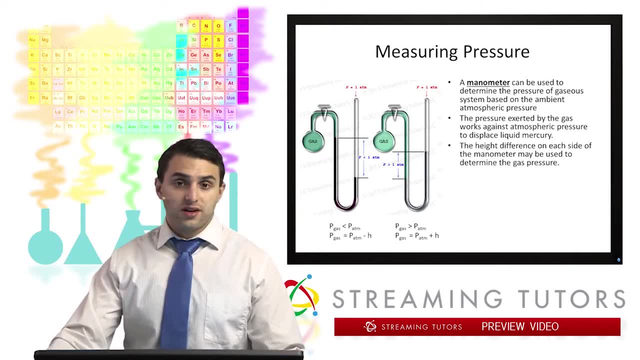 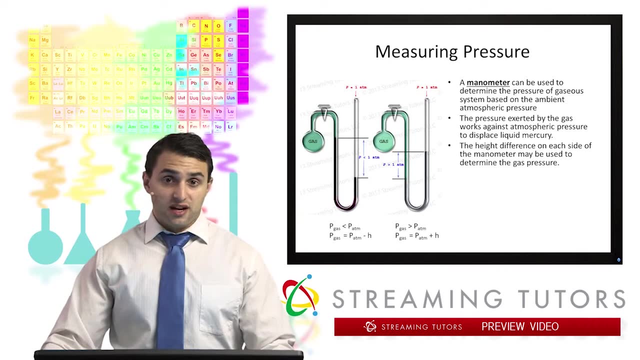 depending on the difference between the atmospheric pressure and the system pressure. So the way that's going to work is, if we have the pressure of our gas is less than the pressure of the atmosphere, we're going to have the pressure of the atmosphere being the dominant pressure, and hence the mercury is going to move towards the gaseous system. 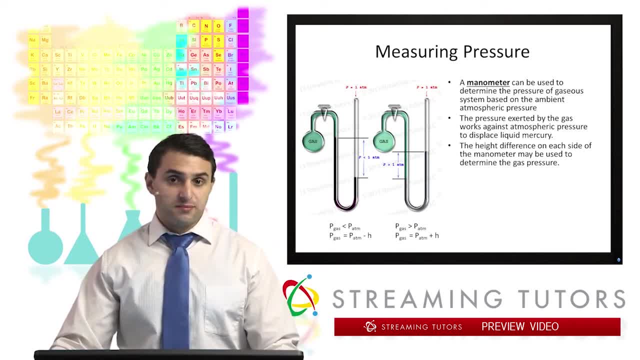 We can calculate the pressure of the gas in that case by just taking the pressure of the atmosphere minus the height difference of the mercury, So that height difference is just the distance of the highest point of the mercury on the left side and the lowest point on the right side of the tube. 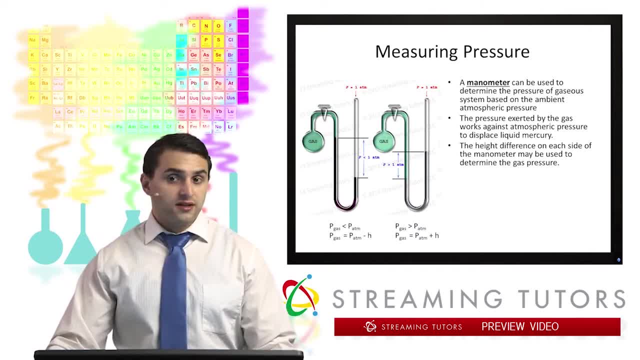 If the pressure of the gas is higher than that of the atmosphere, the mercury is going to be shifted away from the system and towards the end of the tube And we can calculate pressure in that case just by doing the pressure of the atmosphere plus that height difference. 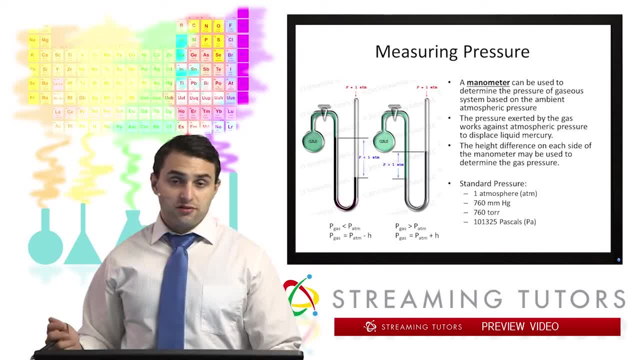 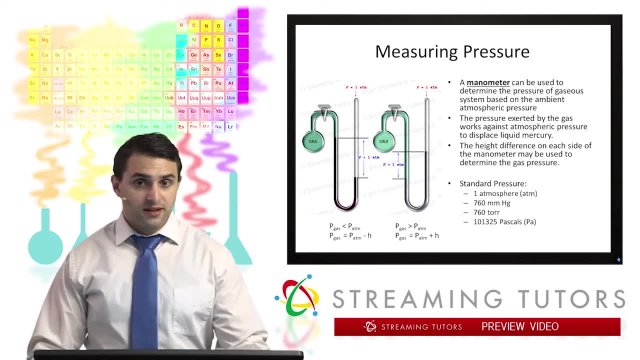 So one other thing to note is that, in general, the standard atmospheric pressure that we're going to be looking at is just going to be equal to 1 atmosphere, which is our most basic unit. That's also equal to 760 millimeters of mercury. 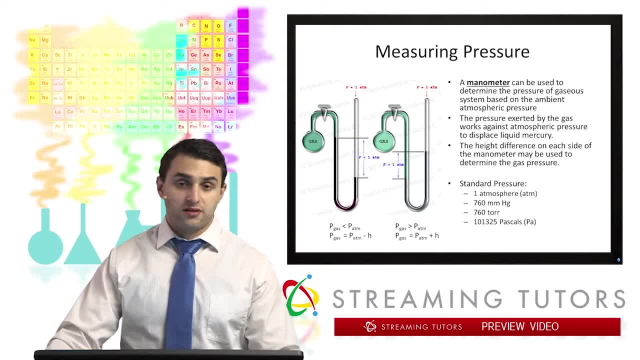 This setup here, Also equal to 760 millimeter, sorry, 760 torr, Or 100,000, and 1325 pascals, Also 101.325 kilopascals, which is probably a common way you've seen pressure on the weather channel or something like that. 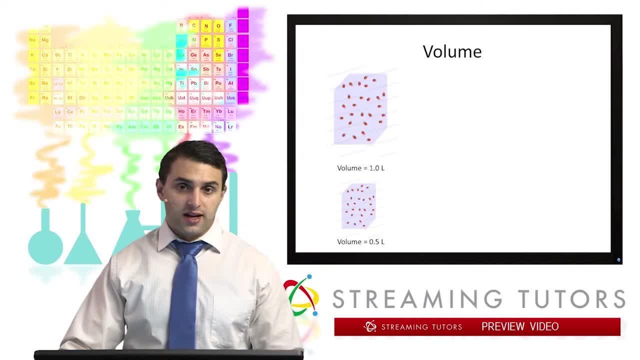 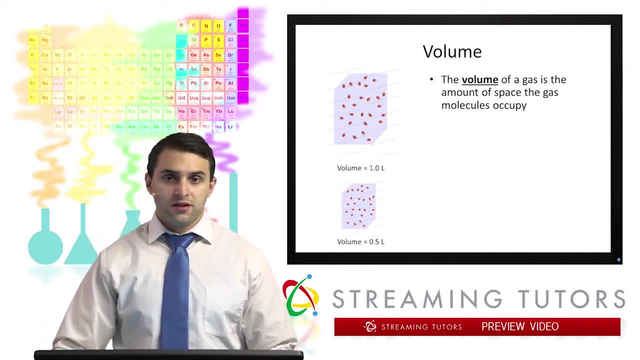 Okay. so next thing we can look at also is the volume of gas. So what happens with gas is, as we know, a gas is going to fill the volume, The volume of its container. So if we put a gas in a large container, it's going to have a large volume. 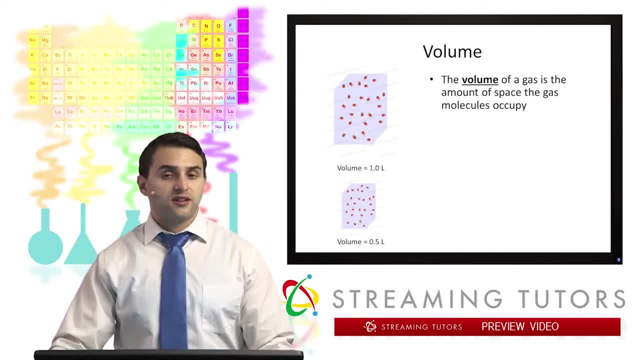 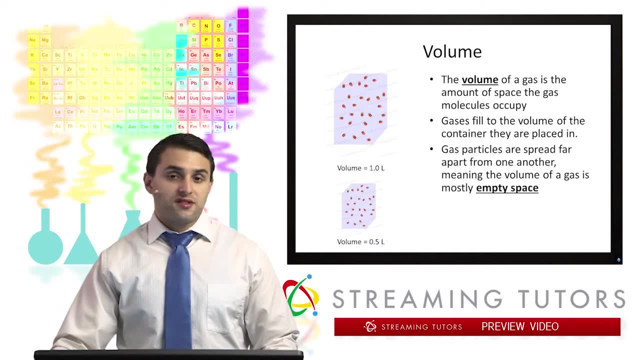 If we have a gas in a smaller container, it's going to also fill that volume, but at a smaller volume. So gas particles are spread far apart from one another in a system, And so what that means is that the majority of the volume of gas is actually going to be empty space in between different gas molecules. 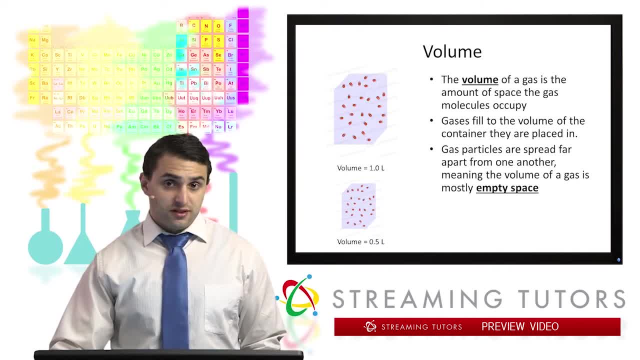 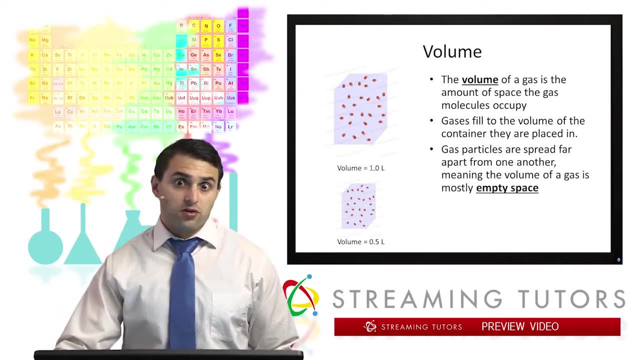 And majority of the volume is just going to be, you know, empty space. What happens also is that when we put the same amount of gas in a smaller container, the pressure is going to be greater Because there's going to be more molecular collisions with the walls in a smaller container. 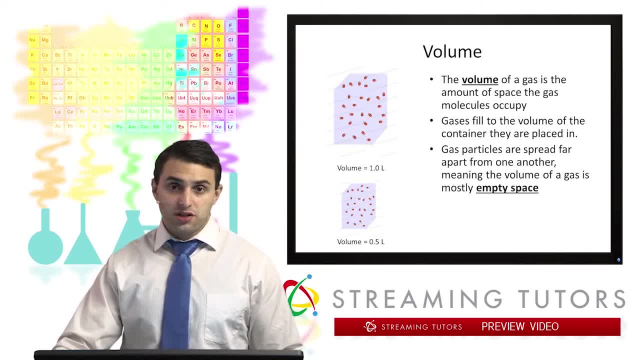 And what we'll see later is that when we have a container that can change its volume, for example a balloon, There's going to be a relationship between pressure and volume. That we'll explore mathematically In one of the later slides. 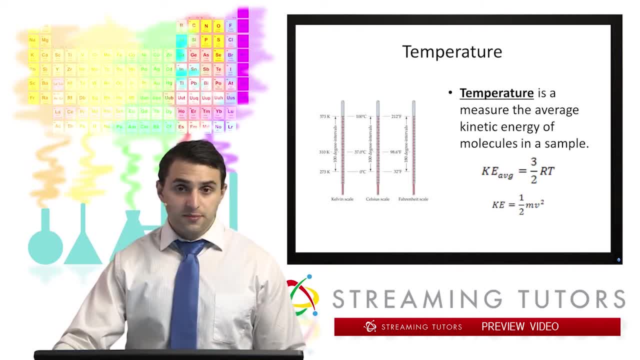 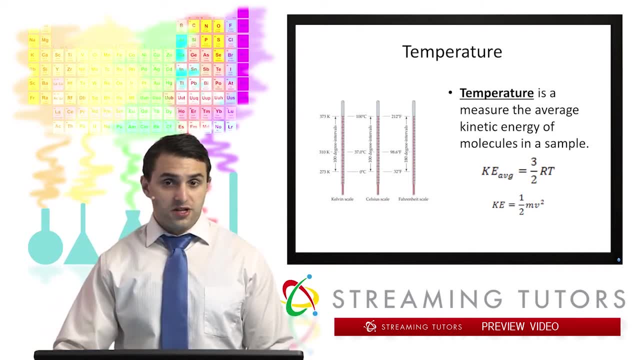 Okay. So then the other thing we can look at is also temperature. We took a brief look at that previously. So temperature, as we said before, is just a measure of kinetic energy of a system. This is a measure of kinetic energy of the gas molecules. 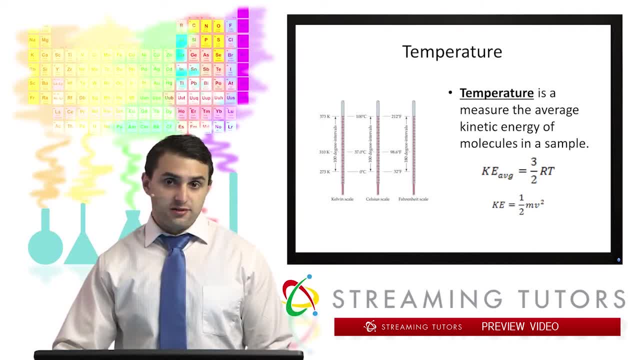 So the average kinetic energy throughout a gaseous system for an ideal gas is going to be 3 halves RT, Where R is just an ideal gas constant that we'll look at later. For an individual particle, The kinetic energy is equal to 1 half mv squared. 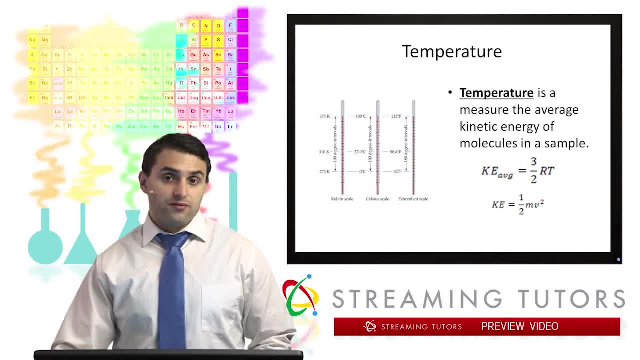 Where m is the mass of the particle And v is the velocity of the particle. So kinetic energy is based on the mass of the particle and the velocity of the particle. And another important thing to know is, as we said before, we're going to be always looking at temperature in terms of Kelvin. 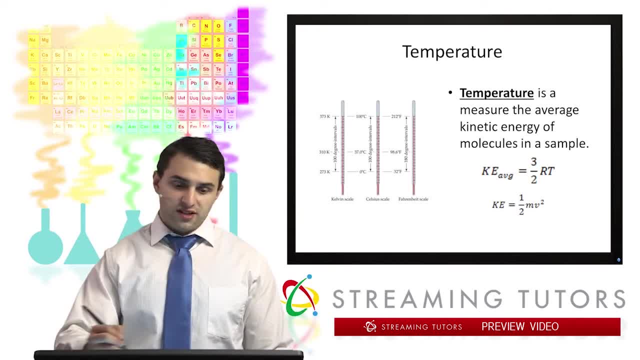 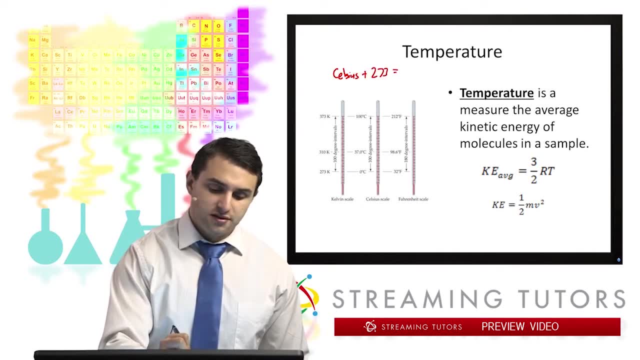 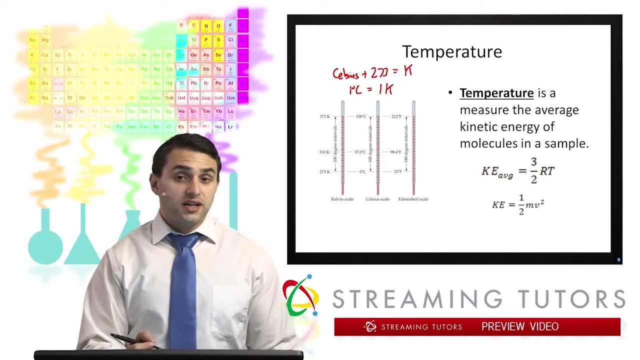 And if we want to convert between Celsius and Kelvin, that's simply going to be that Celsius plus I plus 273 equals Kelvin. An important thing to know, too, is that 1 degree Celsius is equal to 1 degree Kelvin, Meaning if we change the temperature by 1 degree Celsius. 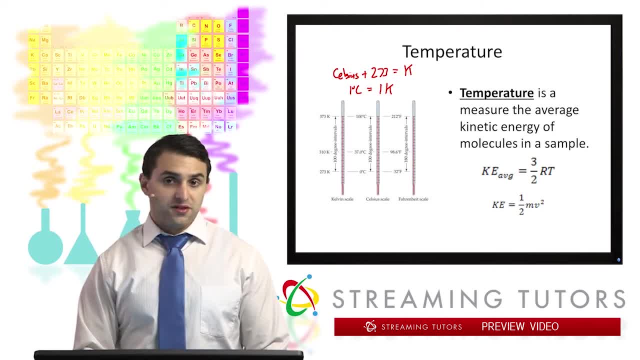 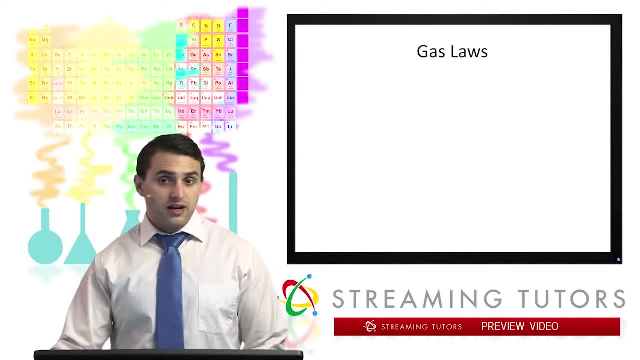 the change in Kelvin is also going to be 1 degree, So in that way they're linearly related, like that. Okay, So now we're going to look at looking at gas systems and looking at them mathematically. So to start with, 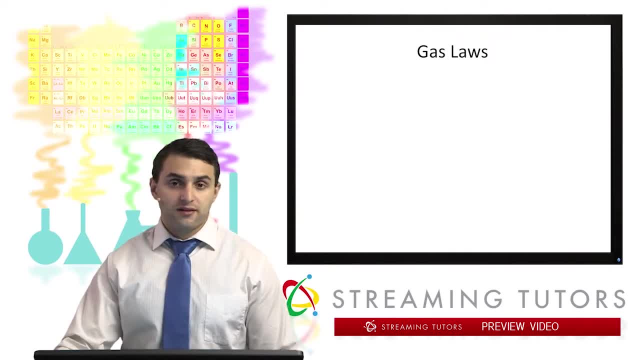 we're going to look at some things called gas laws. These were different relationships that were discovered when chemists were first looking at gases And the relationship between pressure, volume, temperature and the amounts of gas. So the first one is Boyle's Law. 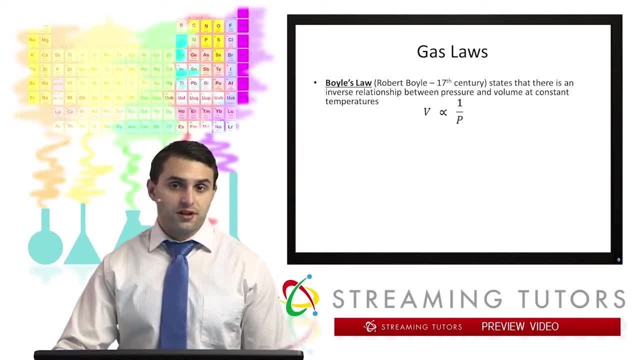 And Boyle's Law states that the volume is indirectly proportional to the pressure of a system. So what that means is that if we increase the volume of a system, we're going to decrease the pressure. That's why we have this here: Volume is proportional to the inverse of pressure. 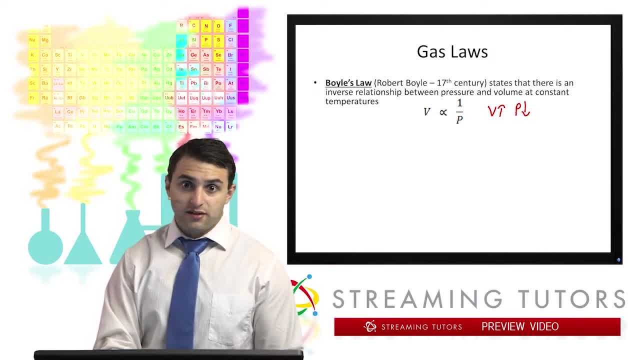 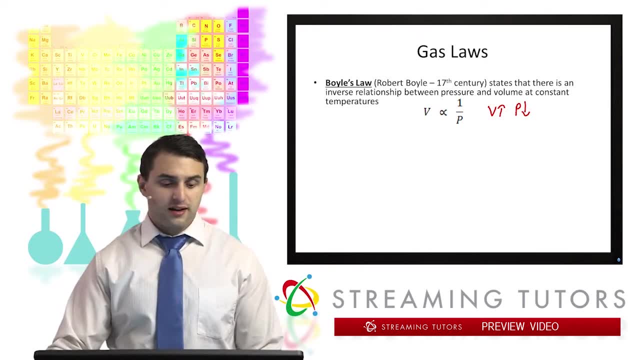 And that makes sense, because if we increase the volume of something, there's going to be less collisions with the container walls, Hence less pressure. The second one we can look at is Charles' Law, And that's just saying that the volume of a system is directly proportional to a temperature. 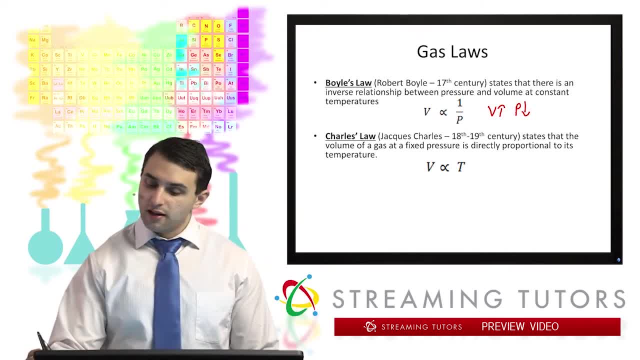 So that means when we increase the temperature of a system, we're going to increase the volume, assuming it's a non-rigid container. And that makes sense too, Since if we increase the temperature we're increasing the kinetic energy of the system, right? 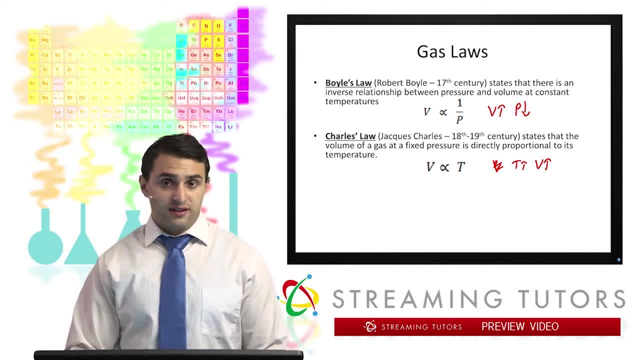 So what that's going to mean is that the molecules are moving more quickly. So that's going to mean that the container is going to expand because there's more energy in the gaseous system. And the last one we'll look at is what's known as Avogadro's Law. 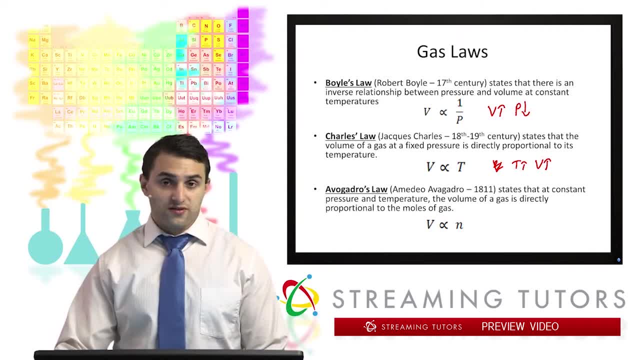 Avogadro's Law just states that volume is directly proportional to the moles of gas, which is pretty intuitive. Obviously, if we add more gas into something like a balloon, then the volume of the balloon is going to increase. Okay, So we can take these three gas laws and combine them. 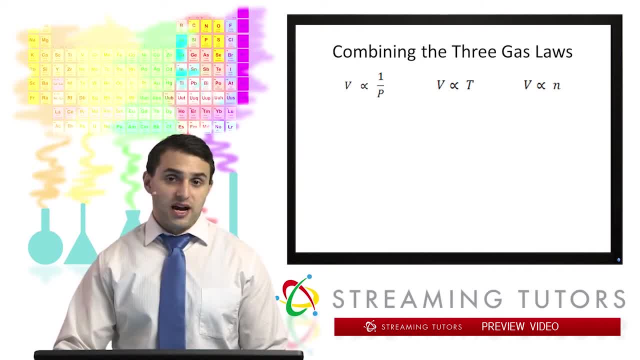 to find a universal expression for describing a gaseous system. So, to start with, if we combine all three of the relationships we just looked at, we can say that volume is proportional to the moles times the temperature over the pressure. So if we want to get rid of that proportion, 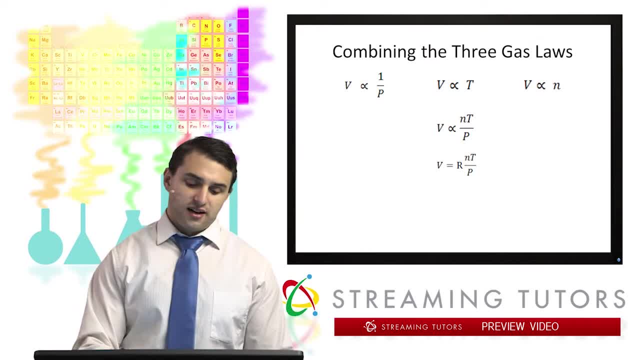 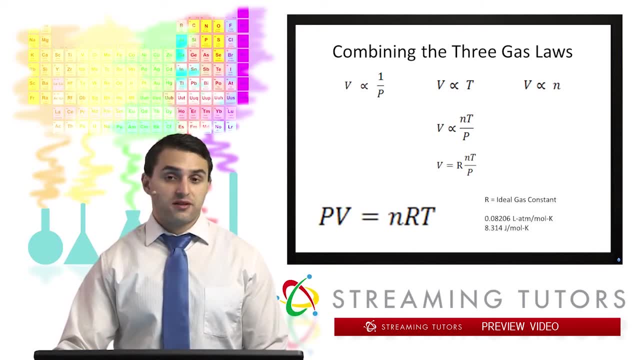 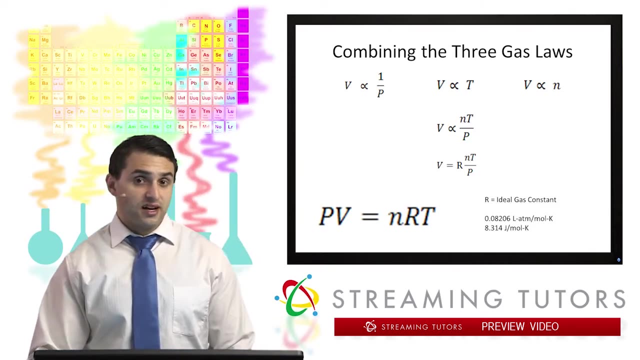 we have to add a constant that relates the two terms. That constant in this case is our universal gas constant R. If we rearrange this, we get the expression: PV equals nRT, That is, the pressure of a system times the volume equals the moles of gas, times R, times T. 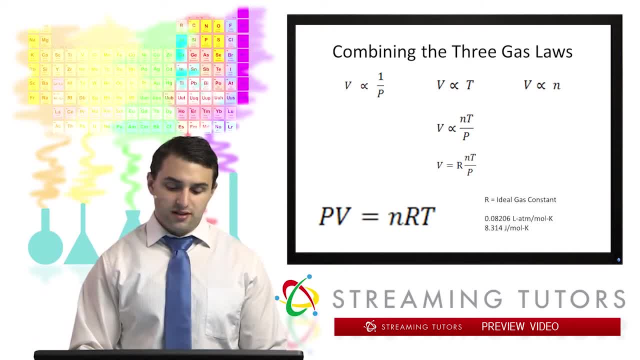 R. here is just our derivative. If we want to get rid of the gas constant, it can be 0.08206 liter atmospheres over mole kelvin or 8.314 joules per mole kelvin. The difference between those is just the units. 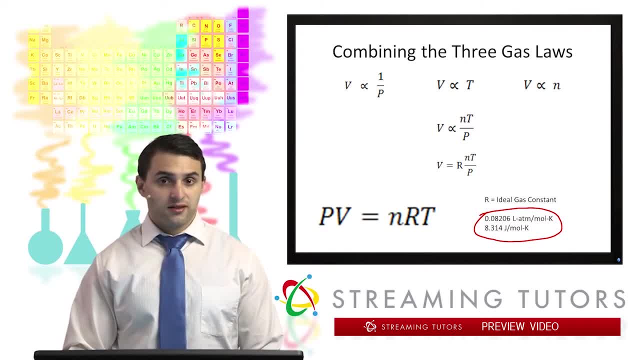 When you're doing your calculations, you're going to want to select the gas constant that matches the units that you're dealing with in your equations. What this also means is that when we're looking at a gaseous system- since we have units of liter atmospheres over mole k-